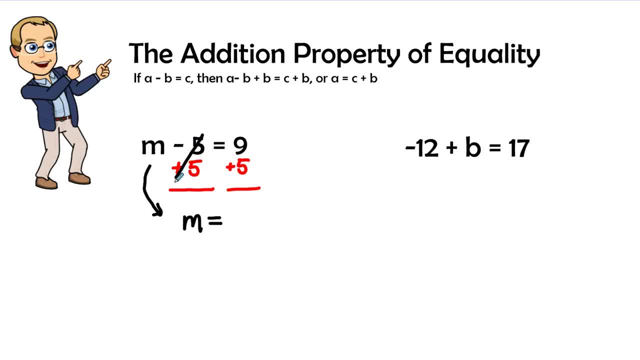 each other, and so that is going to equal zero, And so it would be m plus zero. but we could go ahead and drop that zero off And then nine plus five is 14.. That is just a simple one-step property addition. property of equality. 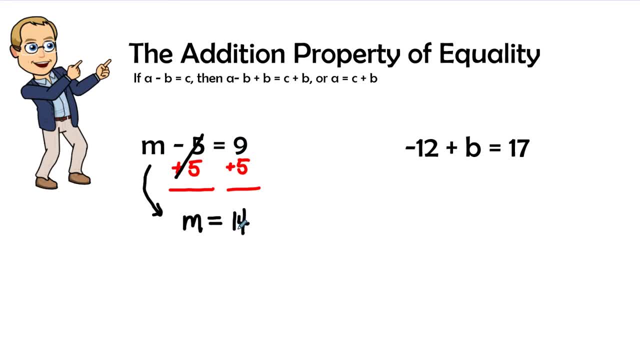 This is also known as a one-step equation. So let's go ahead into the second problem. The second problem. we notice that the variable and the constant are in reverse order. That's not going to be a problem, We will treat it just exactly the same. And so we ask ourselves: 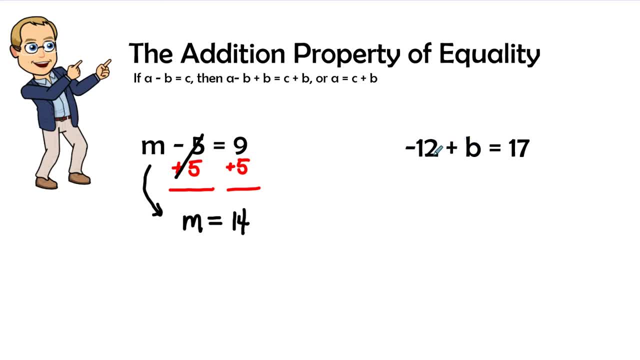 what is attached to the negative 12, or attached to b, And that is the negative 12.. So what is the opposite or the inverse of a negative 12?? It's a positive 12.. So in this addition property of equality, what I do on one side of the equation- 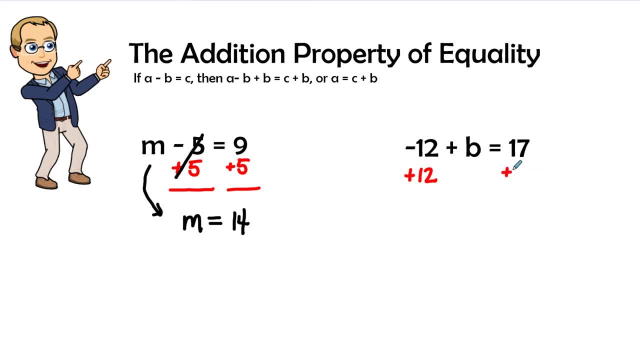 I will do on the second side of the equation, So I'm going to add 12 to the second side as well. Now we go ahead and we realize that a negative 12 and a positive 12 are inverses of each other, And so a negative 12 plus 12 is going to be zero, which brings our variable down. 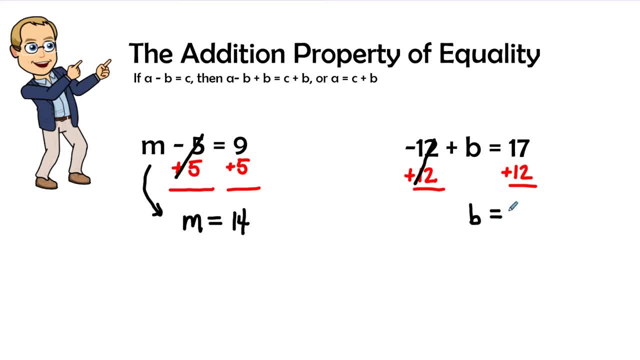 We are going to keep that in mind, And so we're going to add 12 to the second side of the equation. We are going to keep our equal signs in line with each other, And now we have 17 plus 12.. 7 plus 2 is 9.. 1 plus 1 is 2.. So in this answer is b equals 29.. 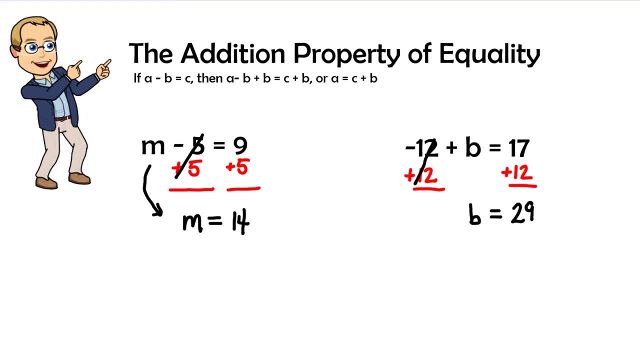 Now I'm going to take another step and let's go back and check our work. So we want to double check our work to make sure it is correct. So wherever I see my variable, I'm going to go ahead and put the number 14.. 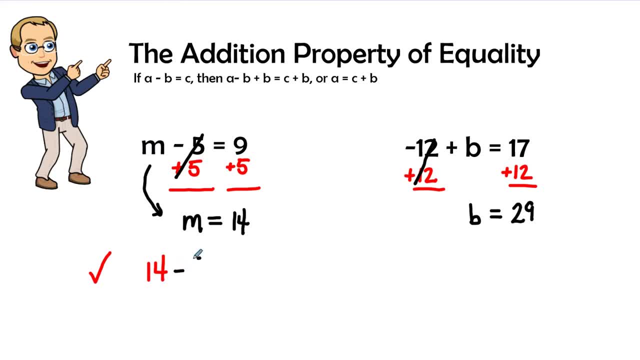 14 minus 5 equals 9.. And 14 minus 5 is 9.. And since 9 equals 9, we know that that is going to check out. Now let's go ahead and see our second problem and see if that checks out. So wherever I see,